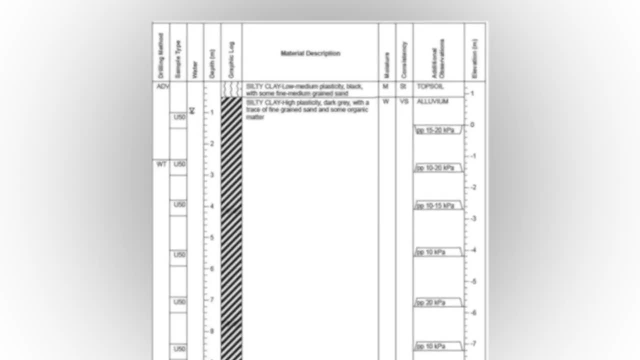 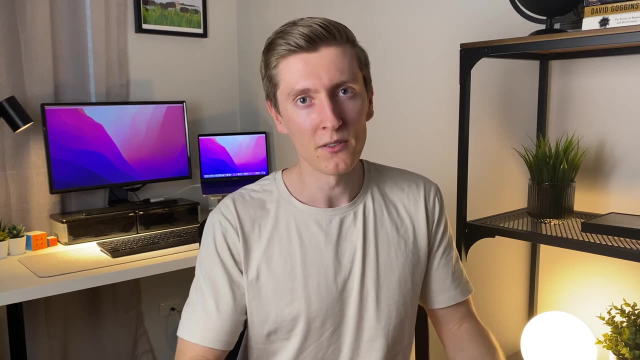 that they can give this soil report to the structural engineers so that they can get an understanding of the soil type, composition and strength, so that they can consider all these things when they're designing the footing system. Alright, so after these three things, 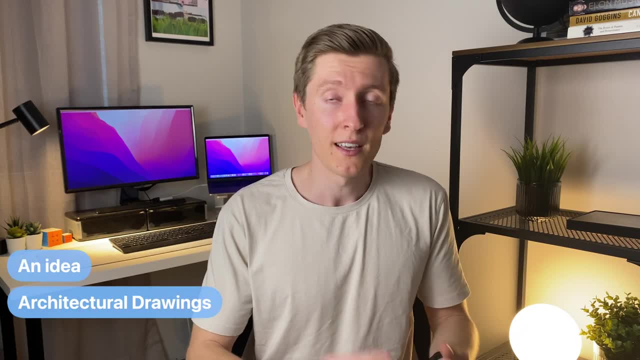 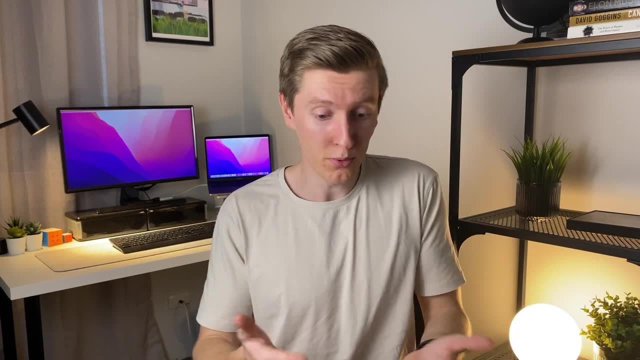 the designer's basically left with three things: They've got an idea, a drawing of that idea and a soil report. And to go any further, this is where a structural engineer will need to get involved, because it'll be their job to figure out how we can turn these pretty architectural. 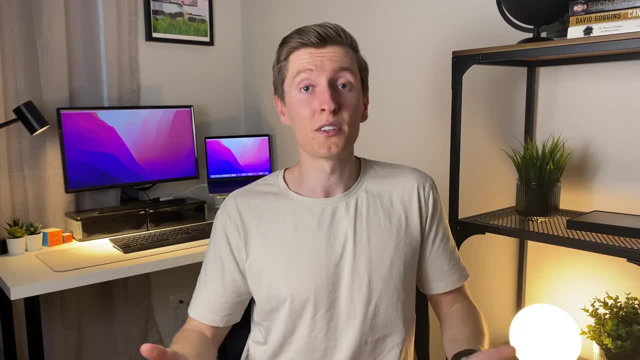 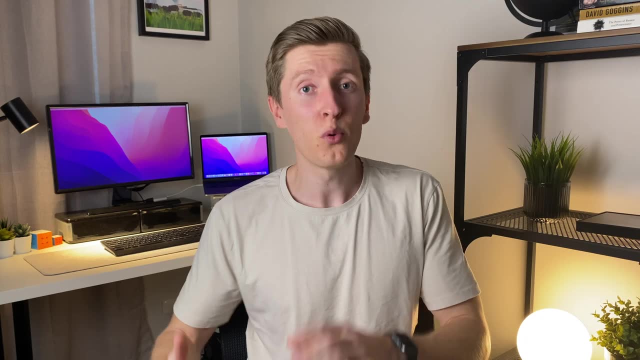 drawings into a strong and buildable structure. So for the structural engineer, this is where the analysis stage begins. During the analysis stage, our goal is quite simple: Here we're just trying to determine all the different loads that a structure is going to experience, so that when 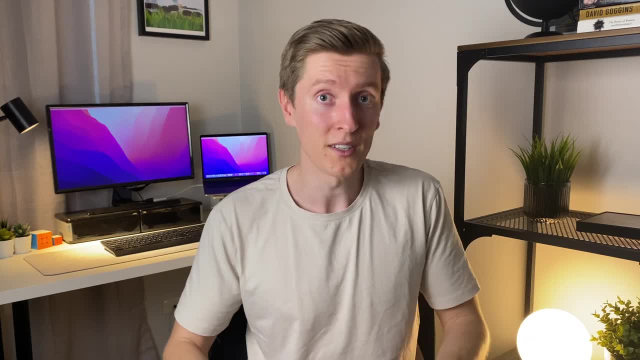 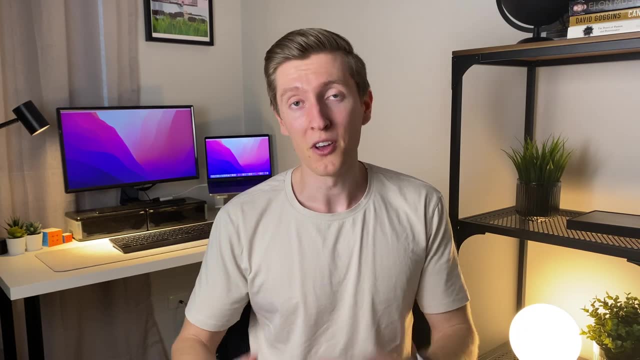 we move to the design stage, we can be certain that the structure that we design can withstand forces and won't fall down or tip over. And, with that being said, there's two different types of loads that we need to determine, and they are vertical loads and horizontal loads. Simply put, 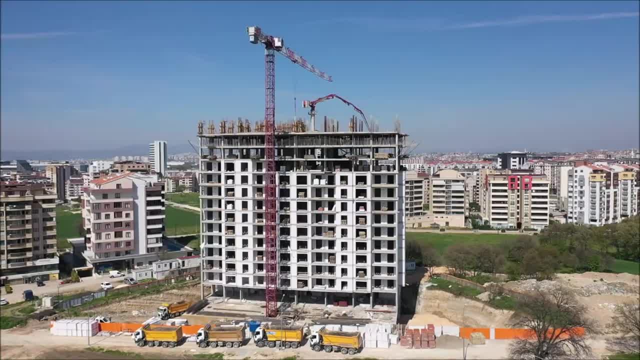 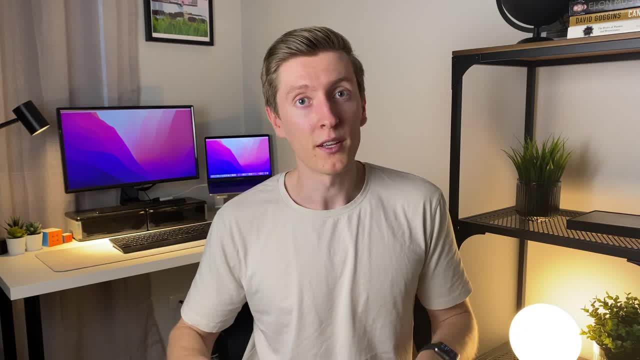 vertical loads are the loads that act downwards, So this consists of things like the weight of the structure itself, any construction materials, any furniture or equipment inside and all of the different floor loads throughout your building. For example, within an office building, you would. 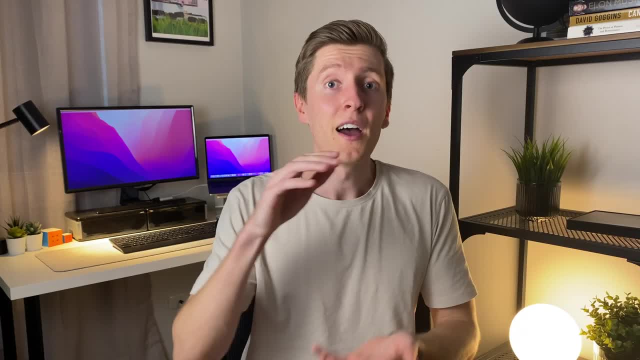 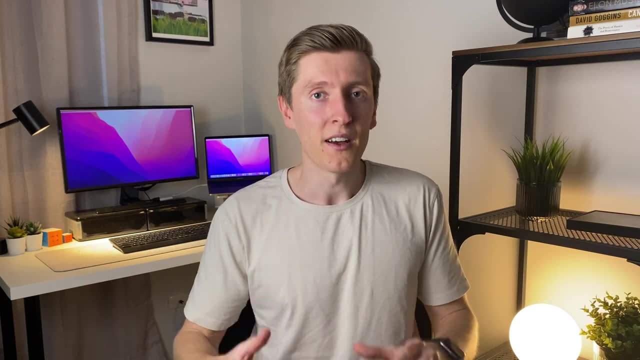 have a certain amount of loading within the general office area, but then a higher amount of loading in places like the storage room, And once we've figured out how big these loads are, they're going to be acting. we then need to design a floor system For an office building. this would 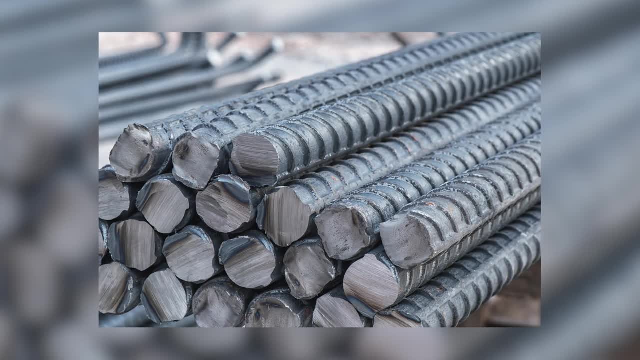 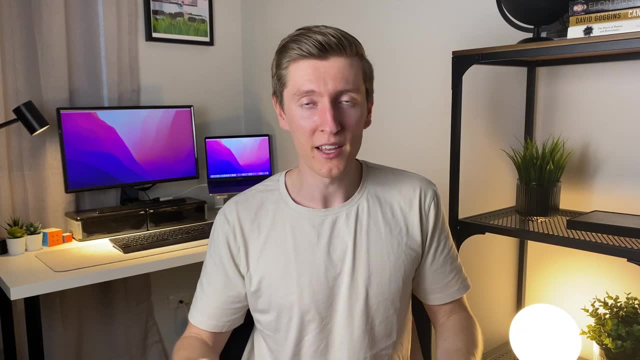 usually be in the form of a concrete slab reinforced with steel bars, and for a house, this would usually be in the form of plywood laid on top of timber joists and bearers. From here, the floor system in the building will then transfer these loads onto the next part of the structural system. 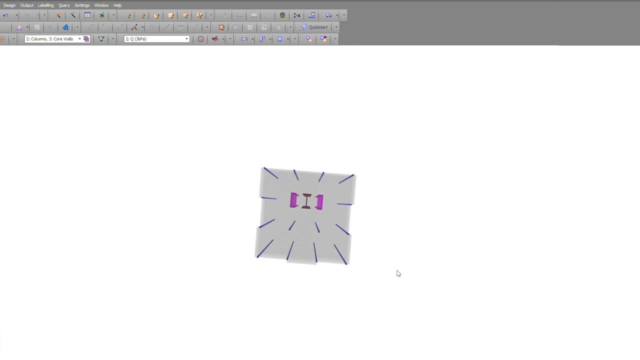 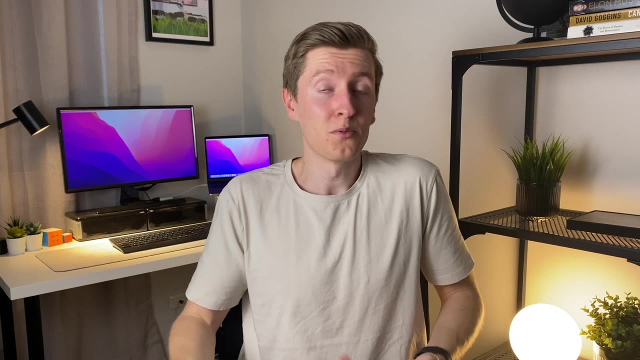 which is the columns and the walls. Now, columns and walls are arguably one of the most important structural elements in any building, because they are the thing that's holding the floor up and, technically, the entire building. If the columns were to fail, everything would come down with it, And besides that, they're also responsible for taking the 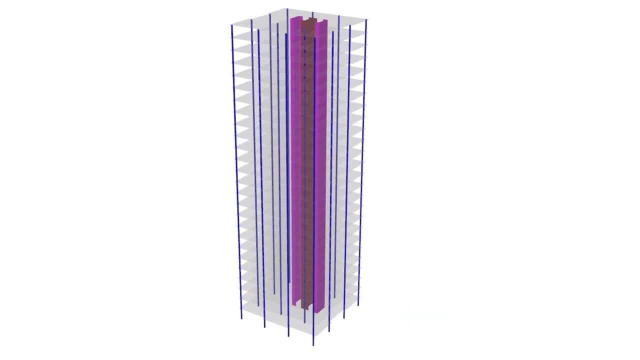 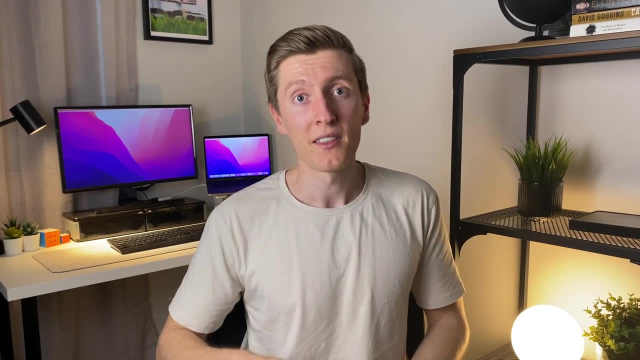 building loads and transferring them onto the next part of the structural system, which is the footings. Once all the building loads have been transferred to the footings, the footings then transfer these loads onto the soil. By completing this load path and getting all the building loads. 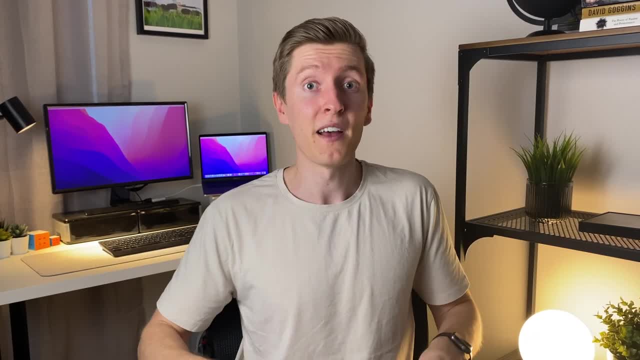 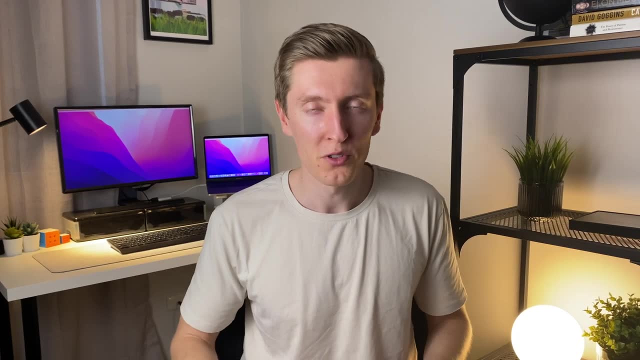 down into the footings and into the soil. that's how we know the building is not going to fail under vertical loads. But that's not the end of the story, because we also need to account for horizontal loads Now, unlike vertical loads, which are applying downward loads on a structure. 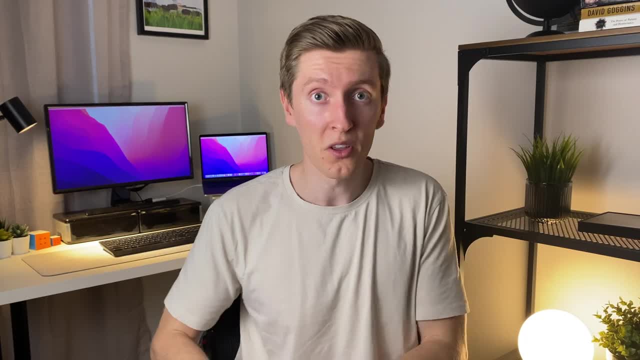 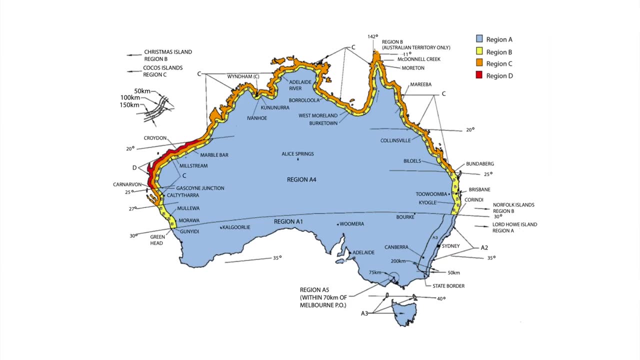 and trying to make a fail in that direction. horizontal loads from winds and earthquakes are trying to push the building over. Structural engineers find out how large these horizontal loads are expected to be from reading national codes and standards, which have often been created from a lot of published research and data on winds. 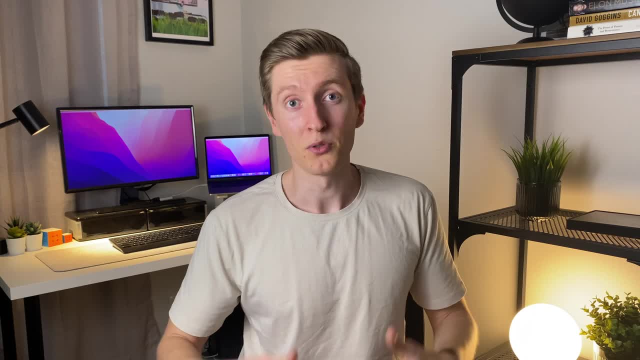 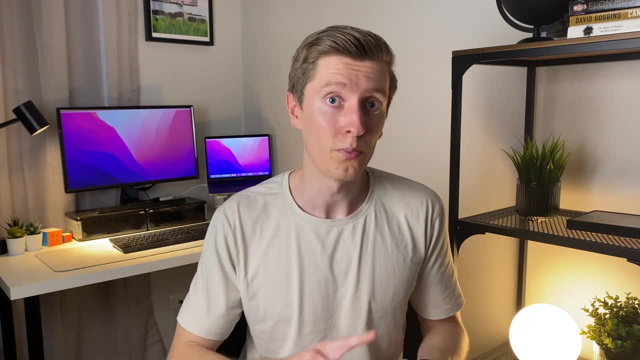 and earthquakes. Now, columns themselves aren't very good at resisting horizontal loads, so we do need another structural system in our buildings in order to resist these loads, and these are often in the forms of walls or braces. For example, in a high-rise building, we often use reinforced 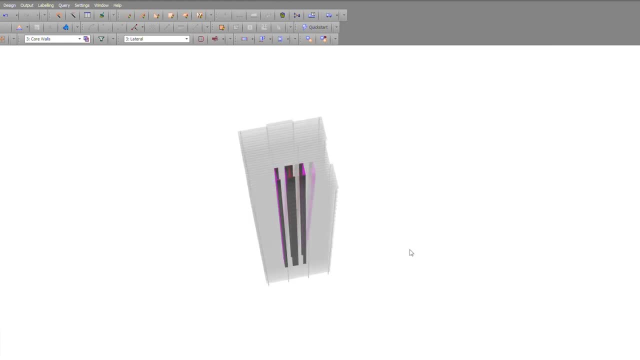 ladders to stabilize the building. These walls basically act as a really long cantilever and are designed so they can withstand the large horizontal forces in combination with vertical building loads. to stop the building from toppling over In a steel frame structure, we often use cross-bracing. 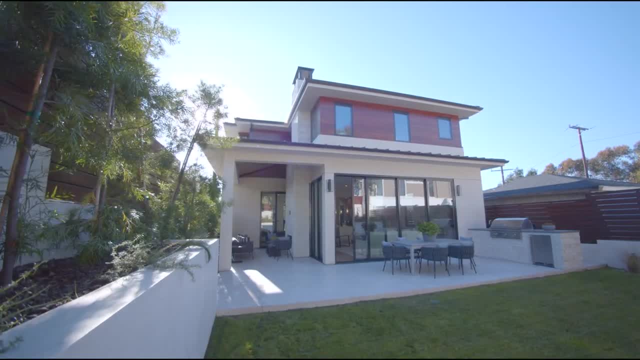 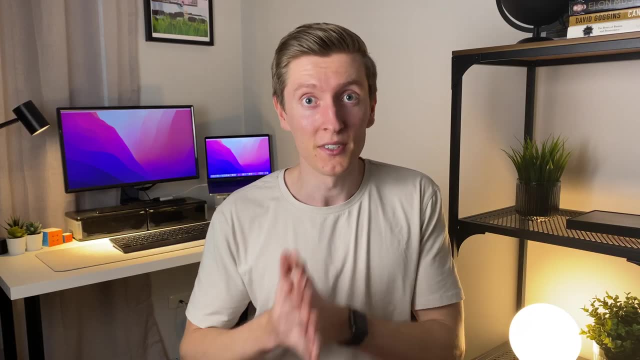 between members, in the roof and walls, to stabilize the structure, and in everyday homes, we use methods such as plywood bracing, strap bracing and power trusses. Alright, now that we've figured out how big the loads are that we need to resist and what building elements are going to be taking what loads. it's time to move on to the design stage. The goal here is essentially to make the building look like it's going to be built from the ground up, and not from the ground up. The goal here is essentially to make the building look like it's going to be built from the ground up and not from the ground up. 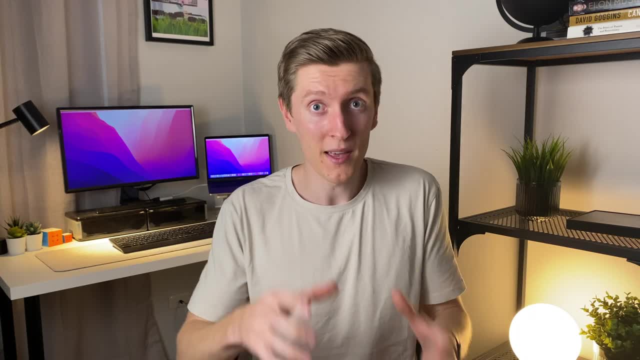 The goal here is essentially to make the building look like it's going to be built from the ground up. The goal here is essentially to figure out how large each element needs to be and how they're all going to be connected. For a high-rise building, this means we need to work out things like how thick the 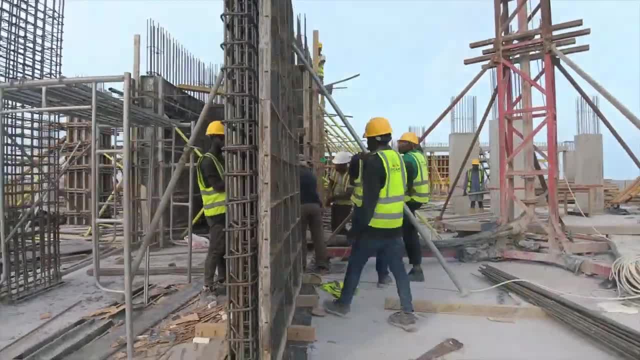 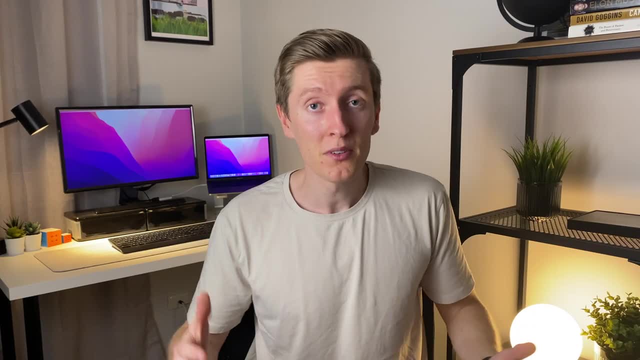 floor slab should be, what size the columns and walls need to be and how big and deep the footings need to go, And we also need to work out how much steel reinforcement is needed in each of these elements. How structural engineers actually go about doing all this is through using their 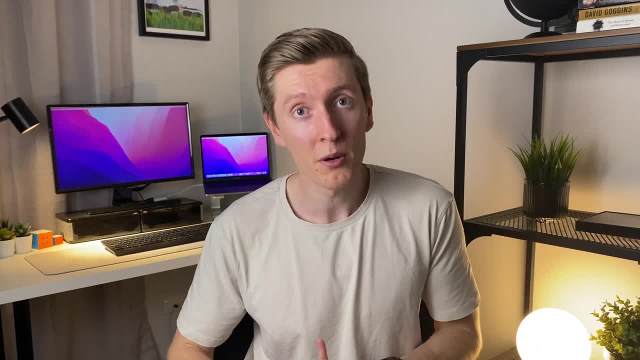 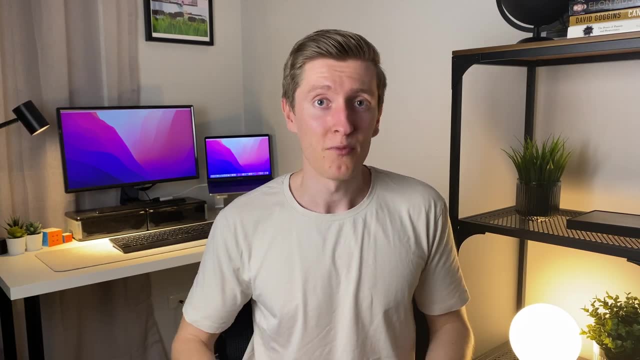 expertise in engineering, mechanics, analysis and material properties that they've learned while they're at university and through many years of experience. Throughout the design stage, we often use a combination of mathematical formulas, spreadsheets, design software and structural analysis models, which all help us to streamline this process and effectively analyze. 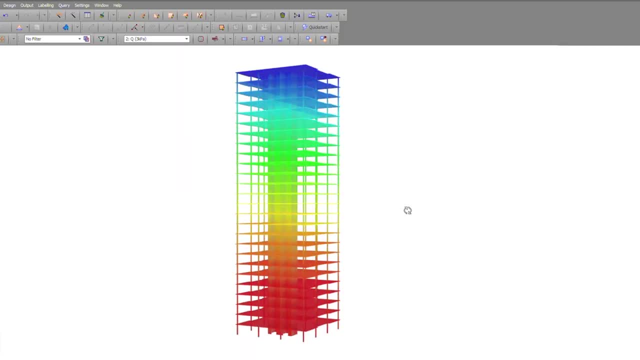 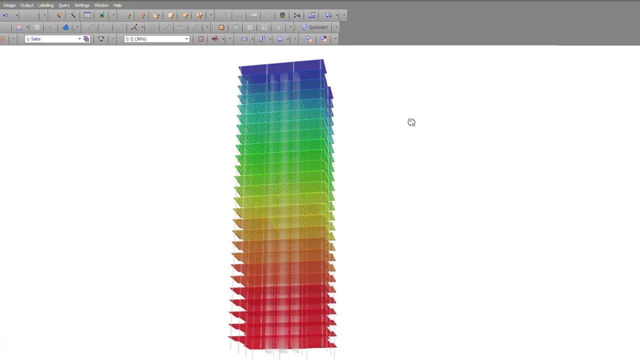 complex structures. For concrete structures like this high-rise building example, often we'll use finite element analysis programs which allow us to model plate elements, because here we can easily see which areas are highly stressed, so we can pay special attention and make sure our design is. 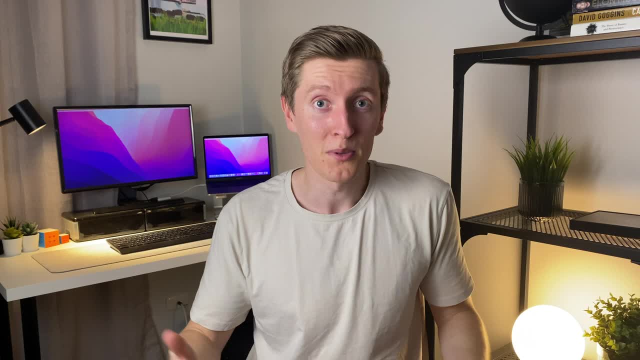 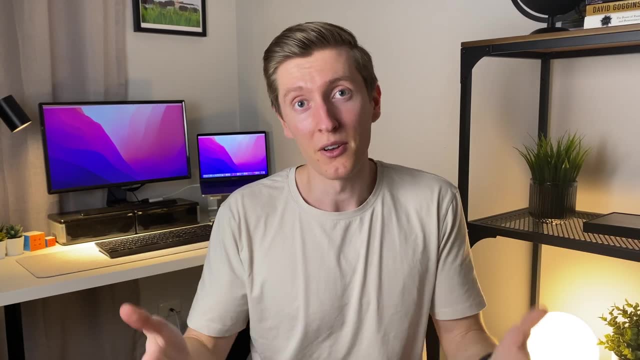 adequate. Likewise, using these same models, we can also look at things like deflection and displacement and so on And make sure that the building doesn't move too much horizontally or vertically under certain loads. Alright, and after the design stage is complete, we then move onto the drawing stage. 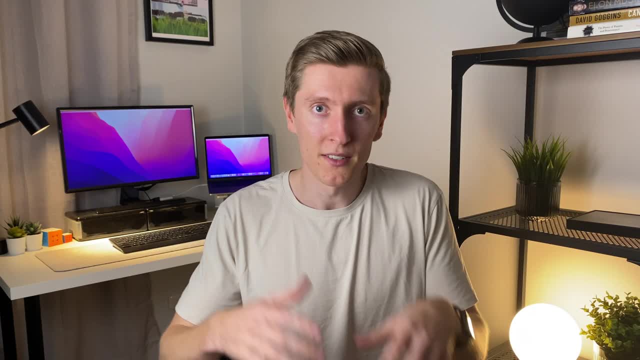 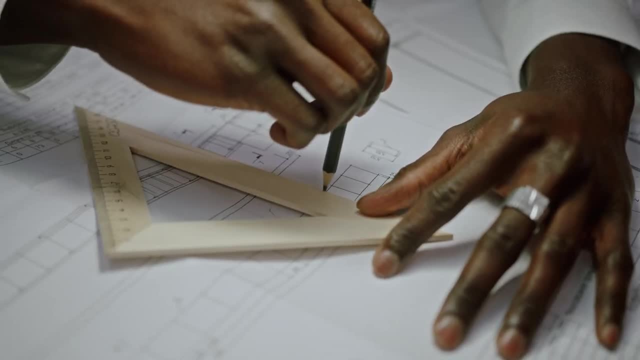 Currently, the engineers have their designs within their calculation pads and software programs, but they can't just give those to the builder and expect the builder to know what to do. Instead, what they need to do is nicely illustrate their design onto paper. Within structural engineering companies, there's usually a whole drafting team whose job it is to 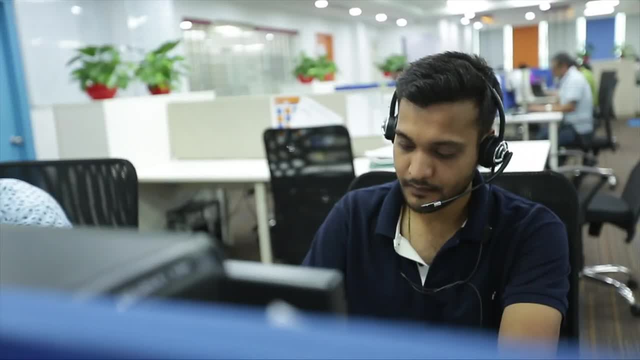 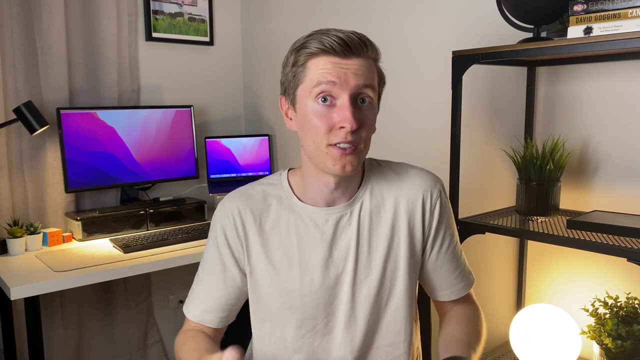 produce structural engineering drawings, and how this usually works is that the engineer will roughly sketch out their final design and the drafting team will take this sketch and turn it into a nice and neat drawing ready for construction. The types of things that are usually included on these drawings are things like the structural element, layout, the reinforcement. 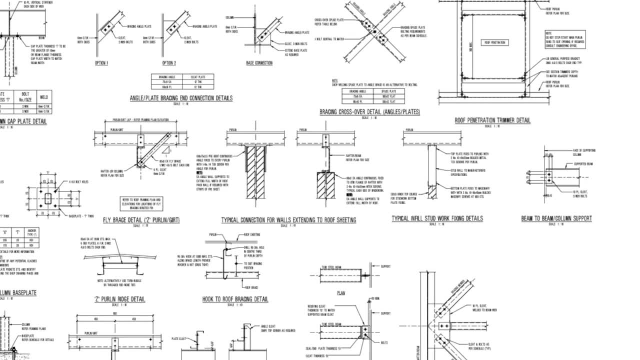 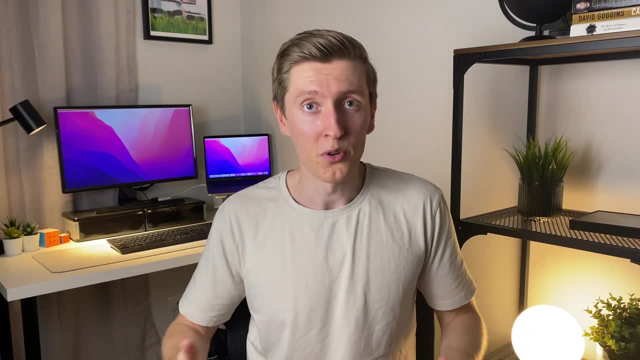 size, spacing and type and lots of other pieces of information which is important to make sure the building is stable and buildable. Okay, and next we have the construction phase. At this point in time, the structural drawings have been checked, reviewed and finalised, and things on site can get started. 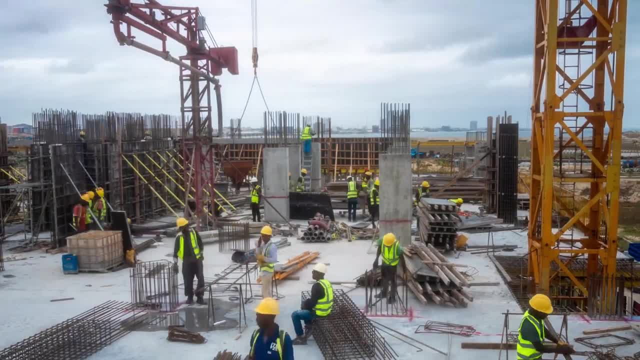 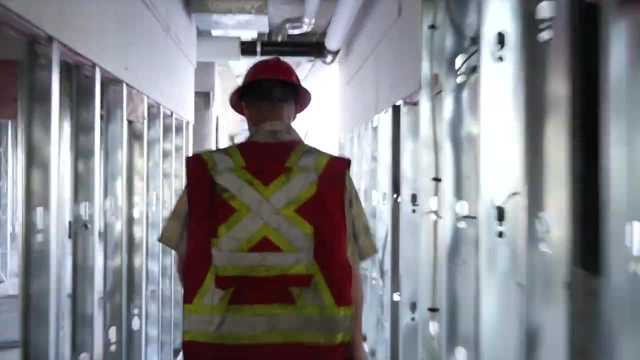 Now, structural engineers don't actually build the final product. those people are the builders or the contractors, but they do actually play a crucial role throughout construction. At regular intervals they will go out to site and do site inspections and make sure that things are being built the same way that they've been designed. 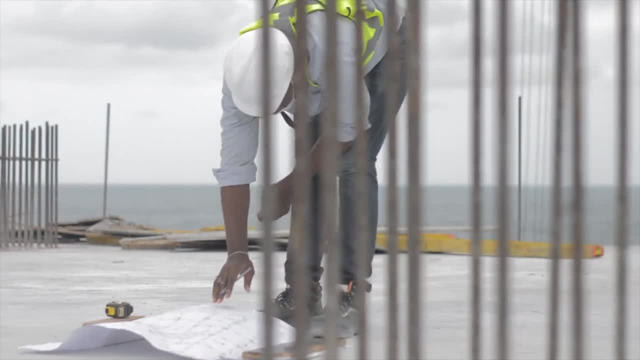 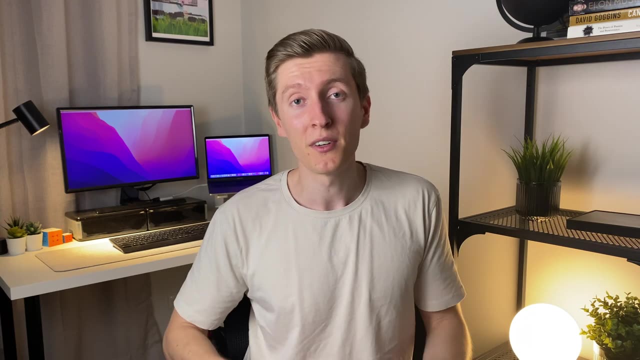 At this time the contractor may also ask them questions and the structural engineer will try and answer those questions to try and help with the actual building. Often things change and mistakes happen on site and the structural engineer will need to come out and provide a solution for when this happens, For example, when the 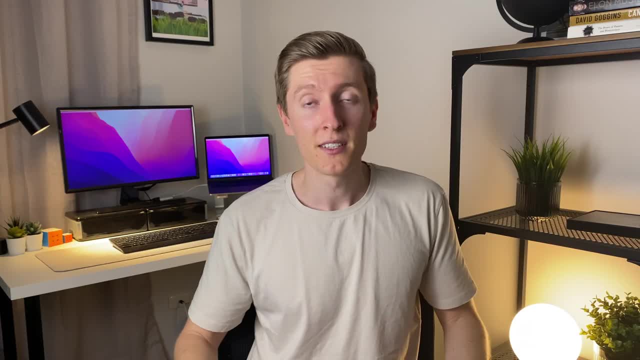 structural engineer is conducting those site inspections, they may notice that the contractor has used 12mm bars where 16mm bars have been specified and in this case they may recommend that they just double up the amount of 12mm bars they've used so that the same amount of 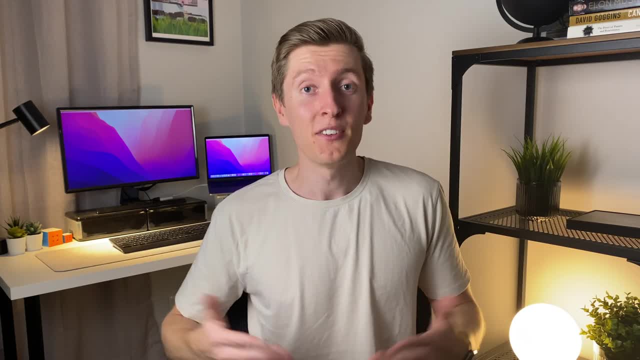 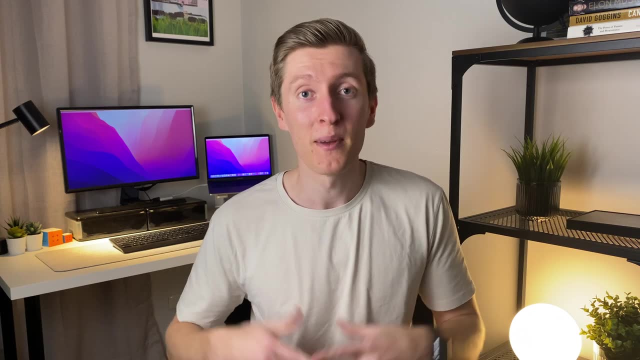 steel is achieved. Anyways, I hope you learned something from this video and if you did enjoy it, you might like this video here where I talk about how I would learn structural engineering if I were to start over, or that video there where I talk about how to make a structural